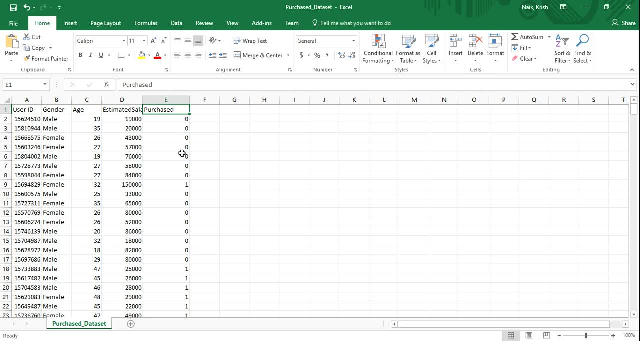 salary, we are going to predict whether the person is purchasing or not. So this is also a different kind of classification problems. What we will do is that we will try to use two different kind of classification problem, and then we are going to use cross-validation. 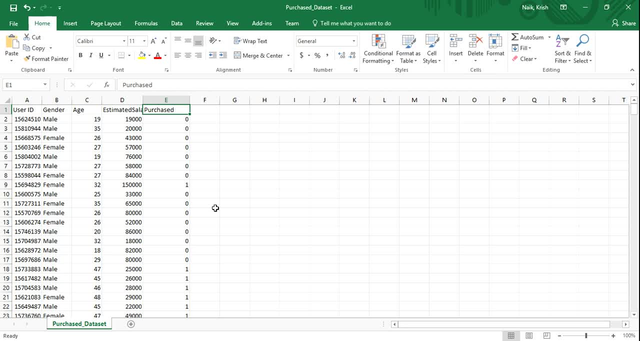 to determine which classification problem is the best for this particular machine learning technique and this particular data set. So you can see over here we have different features like age, estimated salary and purchase. I can also take gender as my independent feature, but I don't want to include the third variable right now. If you want to include it, you. 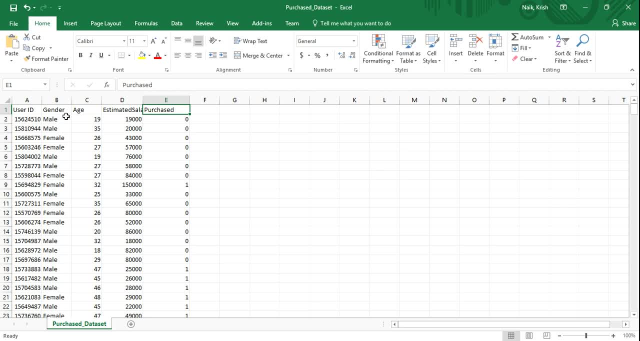 make sure that you convert this male and female into category variables like zero and one. Don't worry about this particular data set. I will be uploading it in my GitHub link and providing the description in the particular description of my YouTube video. So let me. 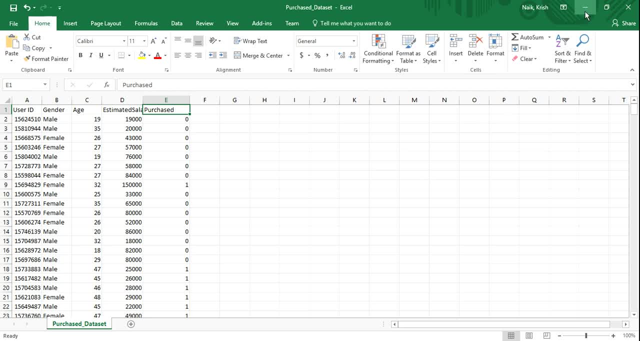 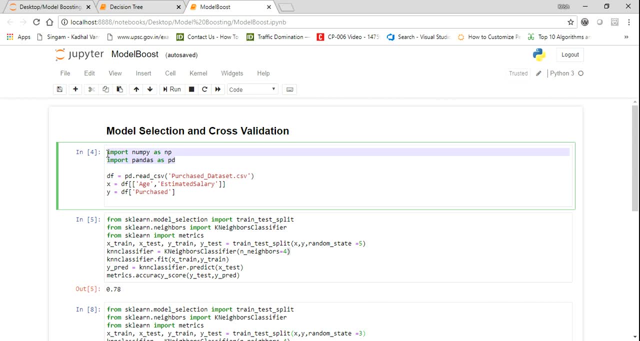 just go ahead and start coding and use this particular data set to solve the classification problem. So to begin with, I'm going to import two libraries, that is called as NumPy and Pandas. I'm going to use read underscore- CSV To read this CSV file. then what I'm going to do is that I'm going to execute the age. 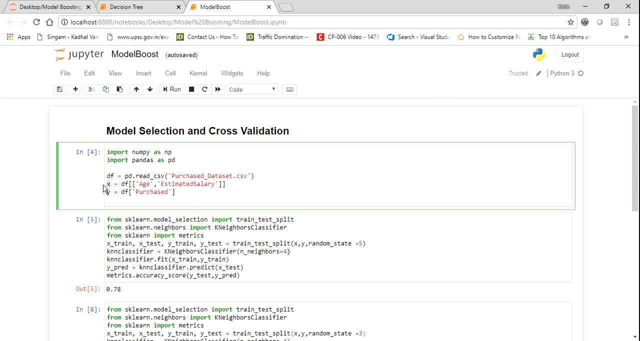 and estimated salary column and I'm going to import it in my independent feature, that is X. Similarly, my purchase column will be in the dependent feature, that is Y. This X and Y will later be splitted into train and test, and then we are going to train our model. 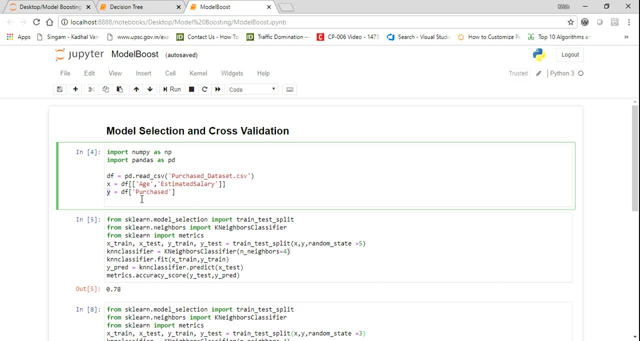 based on the train data and the model I'll be applying to find out the accuracy from the testing. So here it is: I'm going to import the train test split from model selection. Next, I'm going to import the k-neighbors classifier. This is the algorithm that I'm using for classification. 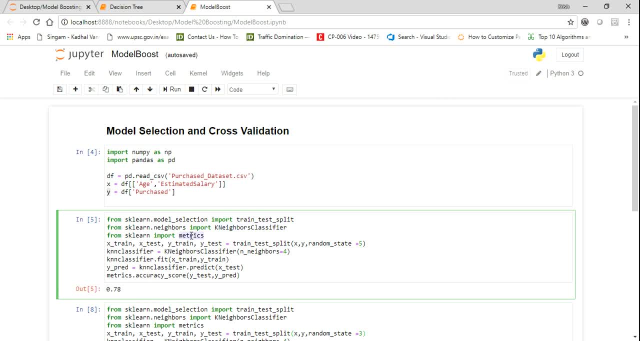 problem right now. After that I'm also going to use metrics. Let me just give a small brief about k-neighbors classifier. k-neighbors classifier is nothing but the k-nearest neighbor which it uses, the concept called as Euclidean distance in the back end. Euclidean distance. 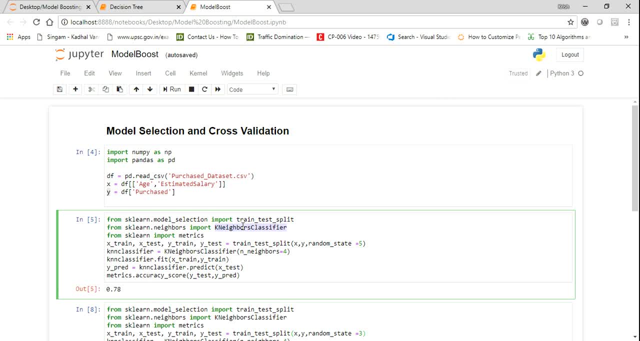 is the distance between two dimension points. Basically, there is a mass formula to this which can be said as root of X2 minus X1 plus Y2 minus Y1 whole square. Sorry, it is also X2 minus X1 whole square plus Y2 minus Y1 whole square, if you are trying to find the 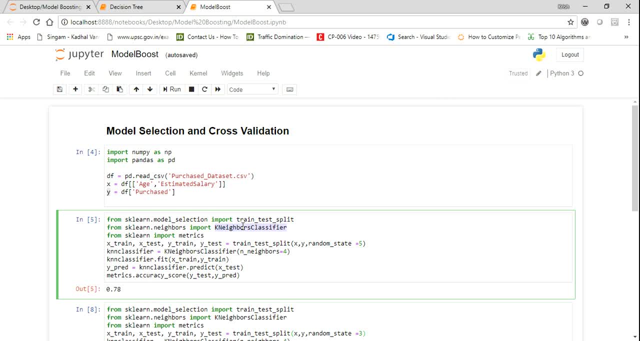 distance between two dimension points. Similarly, with respect to three dimension, the formula changes. So in the next step, I'm going to divide my data set into train and test. I'm using this train and test split library. So I'm going to divide my data set into train and test. I'm using this train and test split library. 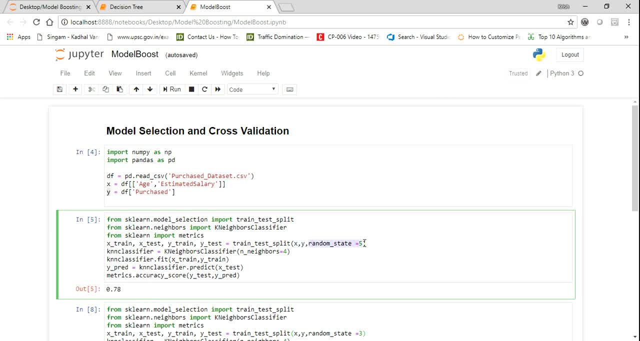 In that I'm giving X and Y and the random state as 5.. Please make a note of this random state value because I'm going to explain about this and how it will be helping us to do the model selection. Then I'm going to call my k-neighbors classifier. I'm going to create 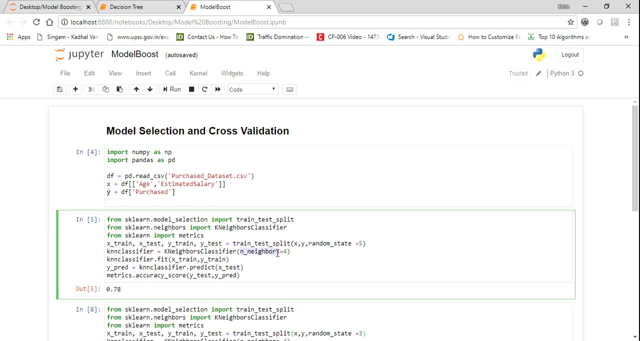 an object, and in that I'm going to consider kn, underscore neighbor is equal to 4.. Instead of 4, I would like to give an odd number, because if I get two nearest neighbors of the three same type at that time it would be very difficult for the model to predict on which. 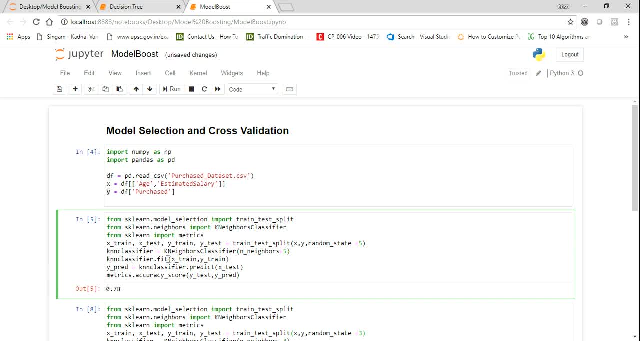 side it has to go. After that, I'm going to use kn classifier dot fit and I'm going to give the X and train and Y train. After that I'm going to predict it and this will be my predicted value. After that, what I'm going to do is that I'm going to find out the accuracy. 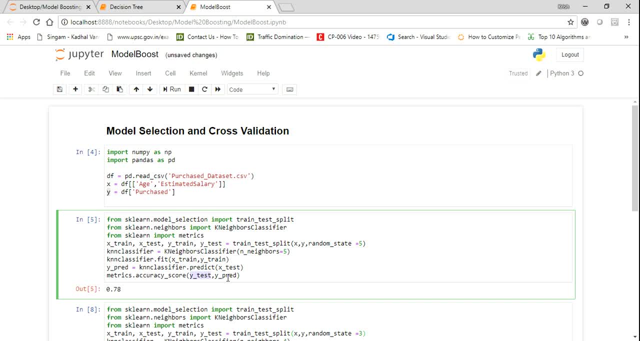 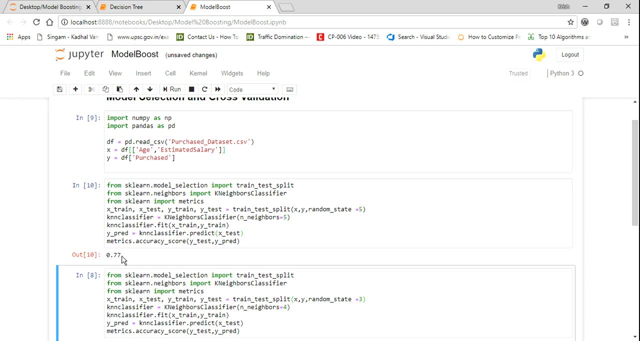 score based on the test data, and I'll be comparing with my Y predicted data. So let me just execute both of this particular line. So it is, I'm getting around 75% of accuracy by kn. underscore. neighbor is equal to 5.. Now 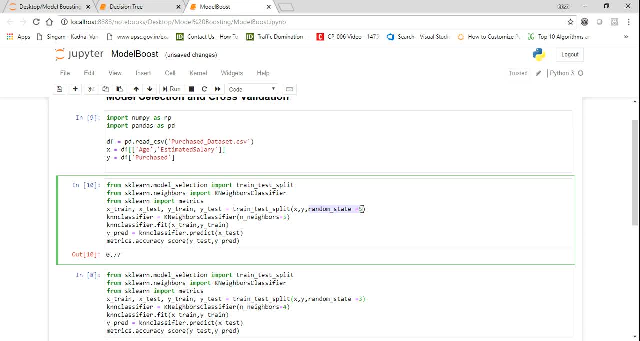 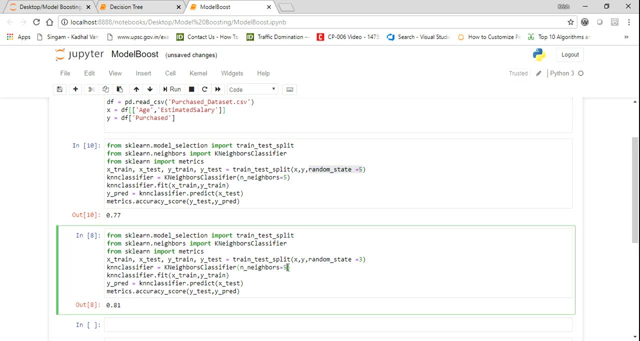 remember that what I told about random state, random underscore state. Now I'm going to copy this code, same code, and I'm going to paste it over here. Remember this: I have made kn underscore neighbor as 5.. Let me change the random state values to 3 and let us see. 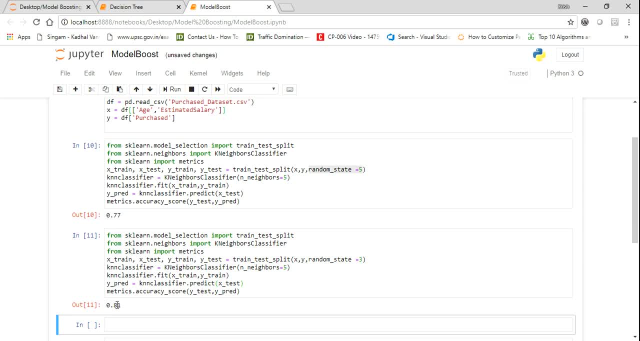 what will be the accuracy? You can see, the accuracy that I'm getting is basically 81%. Similarly, let's change it from 5.. In 1, random state when we are selecting, we are getting an accuracy for 74%. Similarly, 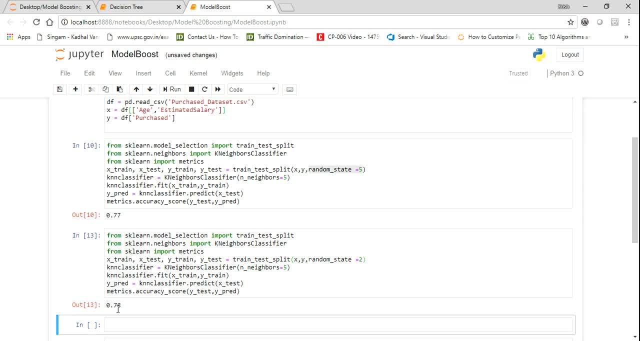 for 2, let's see whether the accuracy will change or not. So it is going to change to 78%. Now let me just play with some more. Like random state is equal to 7.. Now you can see that the value is 0.77, that is 77% of accuracy. Make sure that whenever we are selecting this, 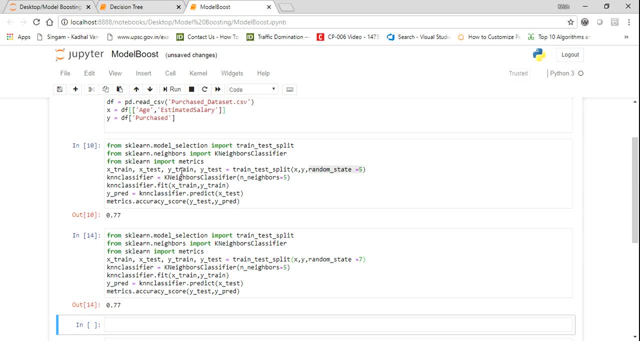 particular random state: the X train and the Y train. that are selected from the random data set that is X and Y. it is selected in a random way. We are just trying to replicate those data and select the X train data and the Y train data together And each and every. 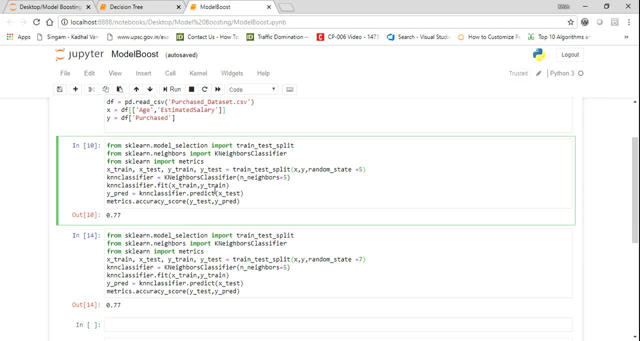 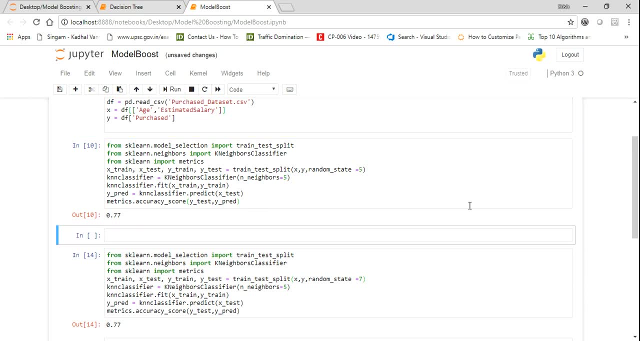 time we change this random state value, we will be getting a different X, train and X test. So in order to see that particular data, let's see how your X, train and X test looks like. So first of all, let me just execute this So you can see that currently, 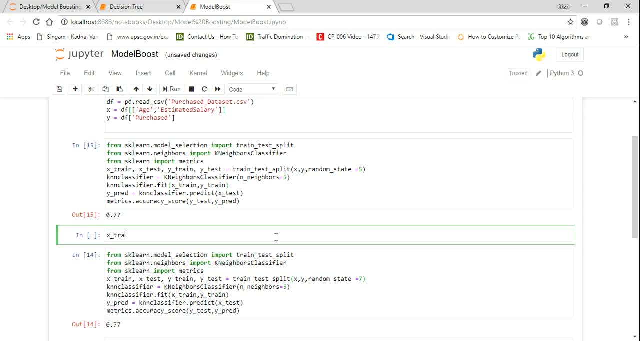 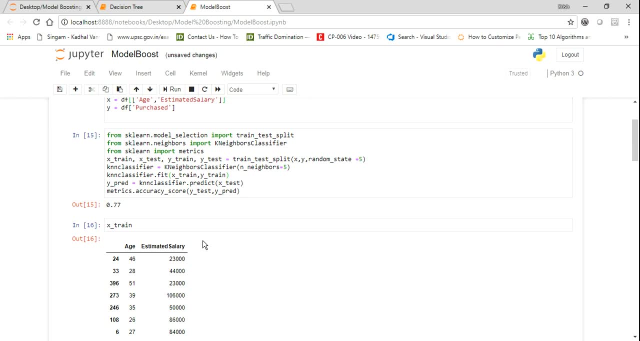 my random state is 5.. Now let me just display the X train value here. Once I execute the X train value, you can see that there are so many values, So let me just write head so that it will just display me the top 5 rows. So here it is. These are my top 5 rows. See the indexes from: 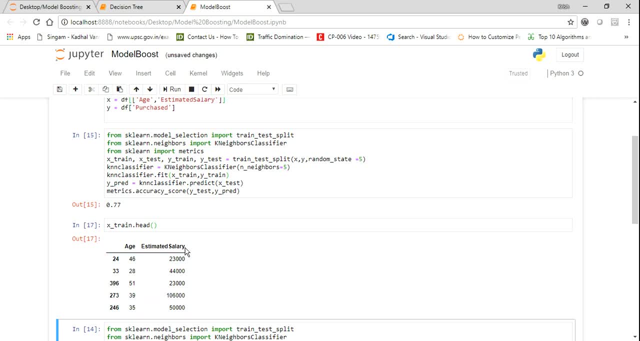 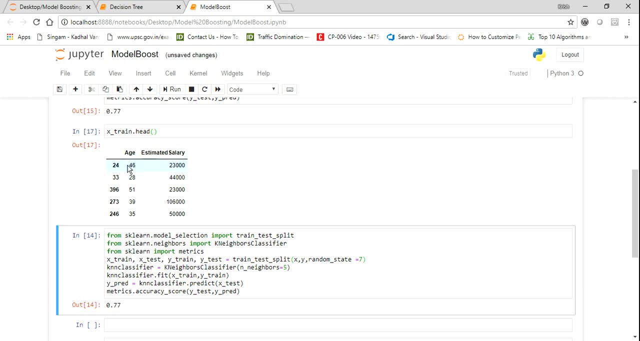 this data base data set. Different indexes are selected and they are combined into train data set. Now what I am going to do is we will be observing the first row over here. Suppose the first row here is 5.. Age is 46.. Estimated salary is 23,000.. Then what we are going to do is that we are going 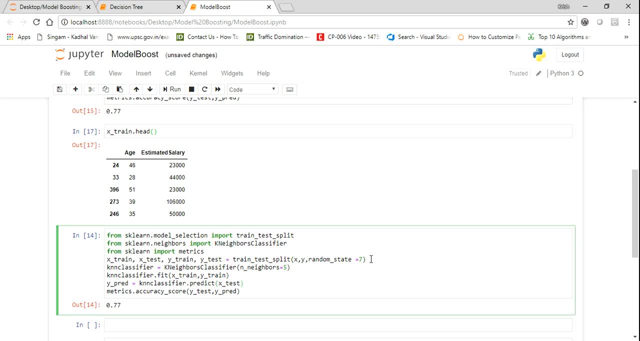 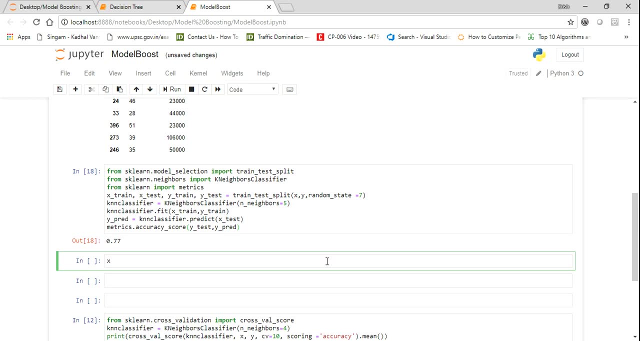 to copy the same code and paste it over here. I am going to change the random state to 7.. So let me just execute it. and what I am going to do is that I am going to see the X value. Now again, I will use Xhead to just see the top 5 rows. Now let us see what was the first. 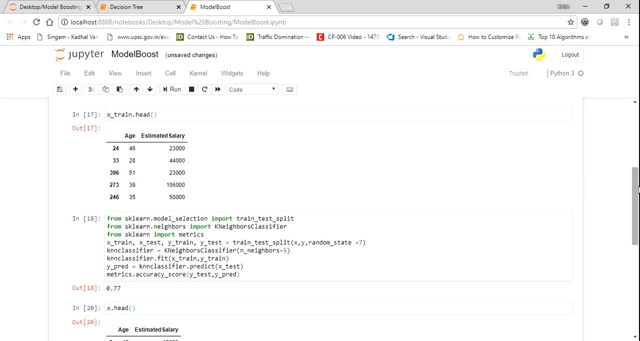 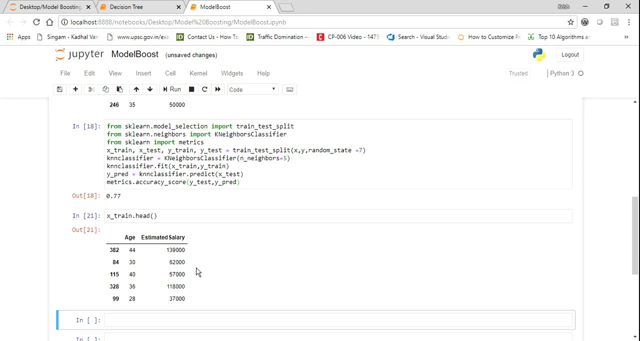 value in the upper X train And what is my lower? sorry I had written X over here Instead. make it as X train. So here it is, X train. Now observe the first value. Age is 44 over here and we have 139,000. 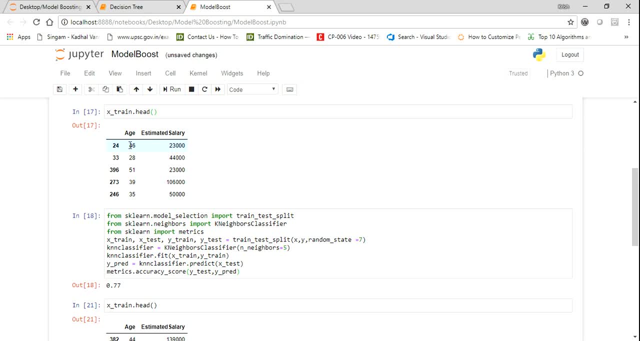 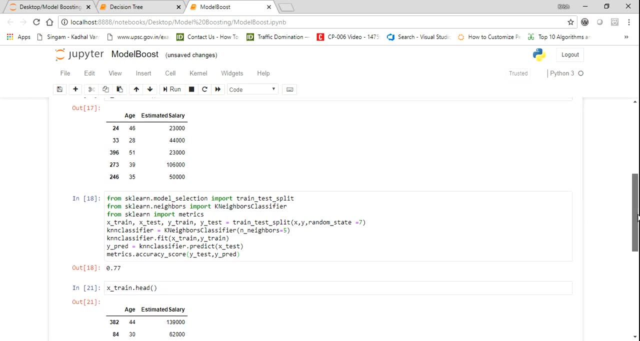 estimated salary. Similarly, if I go first up, my first row is basically: age is 46 and my estimated salary is 23,000.. So what I am going to do is that the conclusion that comes out from this is that if we change, 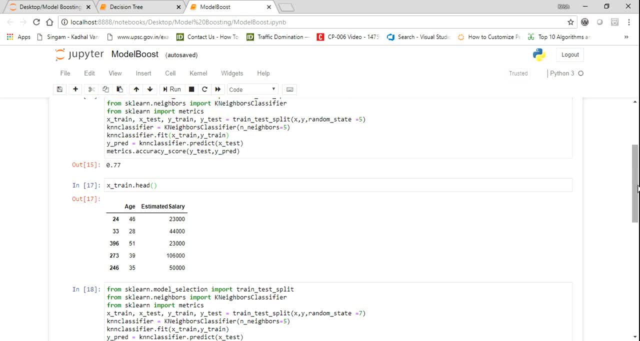 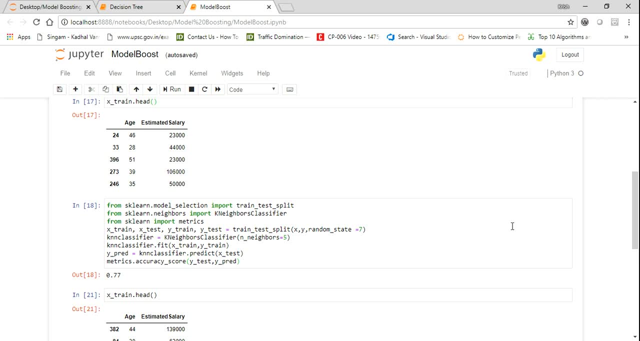 the random state. Then there is a different random selection of the X train and the Y X test data. Similarly, in this case, we are selecting random state as 7.. The X train and Y train data also gets selected in a random way. 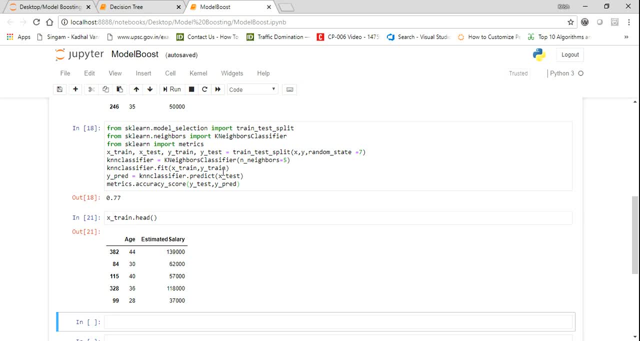 So you can see that as we use different, different random state, there is a chance of changes in the accuracy score right. Sometime it is coming as 80,, sometime it is coming as 70. So let us use this concept in the form of cross validation Now before applying cross. 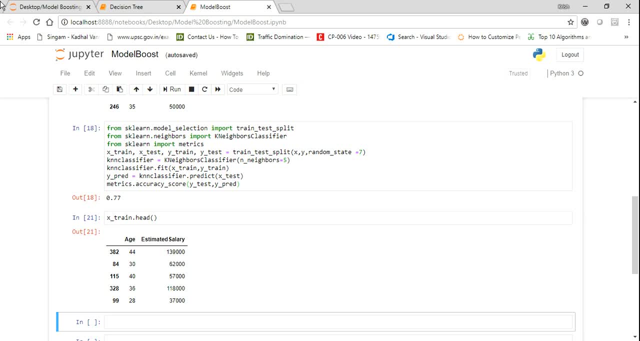 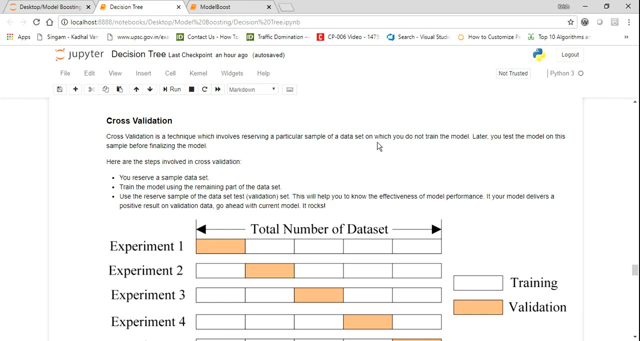 validation. we will be seeing what is what it is. So here's a small diagram of cross validation. Cross validation is a technique which involves reserving a particular sample of data set on which you do not train the model right. Later you test the model on this sample before finalizing the model. 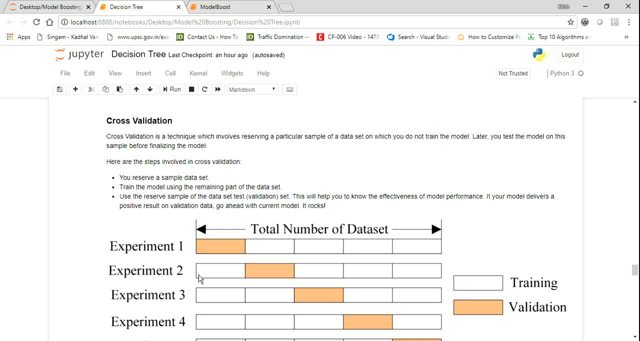 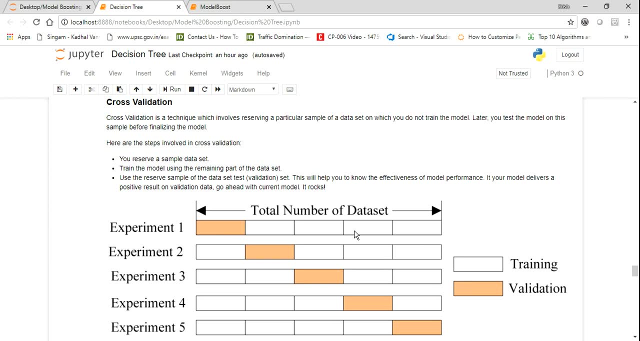 So let us see the steps that are involved in the cross validation. guys, observe this particular diagram. It is very, very, very important. Now suppose you have this 25 set of data. So I have 25 rows of data and I'm treating as one block as 5 data, the other block as another. 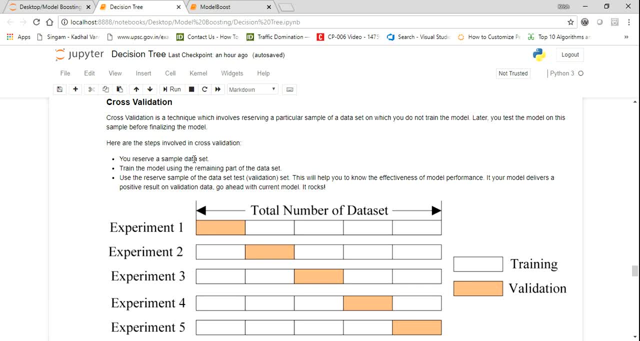 5 data, then 15,, 20, 25.. First of all, you reserve a small sample data set, So suppose I reserve the first sample data set and this particular data set will be used like my testing set. Okay, The remaining data will be basically used by, like my training set. 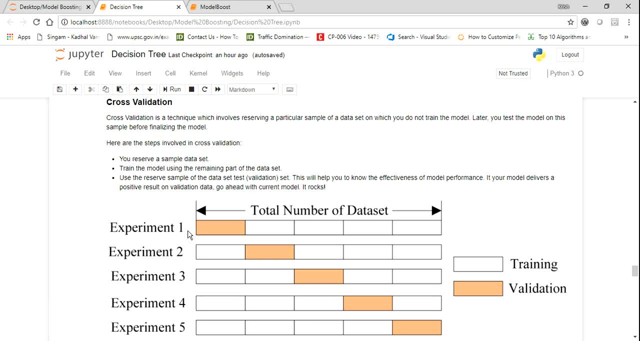 So this will be my first experiment. That is basically my first loop. Then, in the second experiment, what I'm going to do is that my I'm going to second set. I'm going to select the second block as my test data and the remaining block as my training. 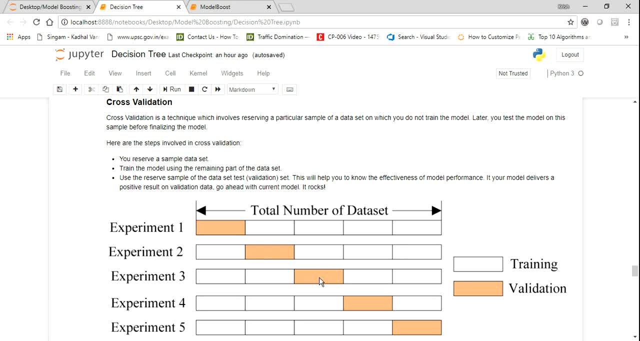 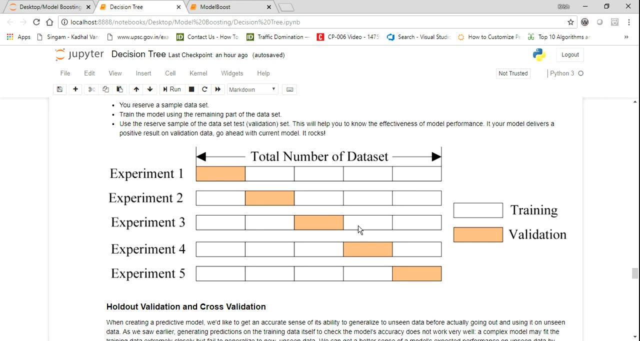 data. Similar in the case of experiment three. I'm going to select the third block as my training data, sorry, as my test data and remaining all data as my training data. Similar in the case of experiment four and experiment five. This way, you can see that we are having different kinds of test and training data. 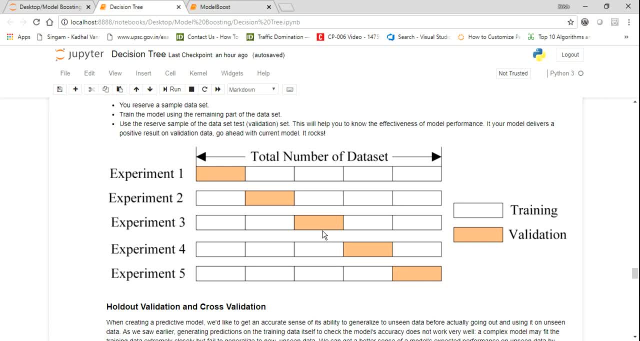 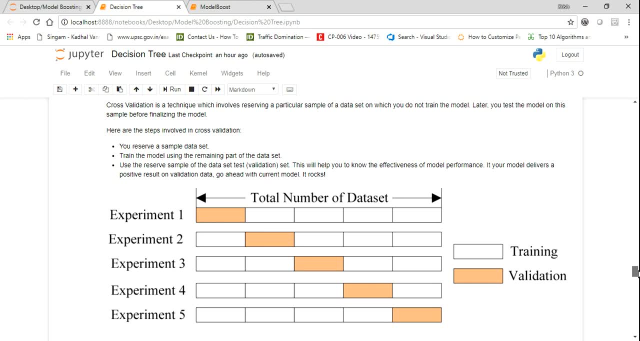 And because of this, what will happen? the model will be able to understand different, different kinds of data, So the model will be able to understand different kinds of test and training data, with respect to both training and test data. So because of this, we may get a better accuracy and the model will be able to deliver a very 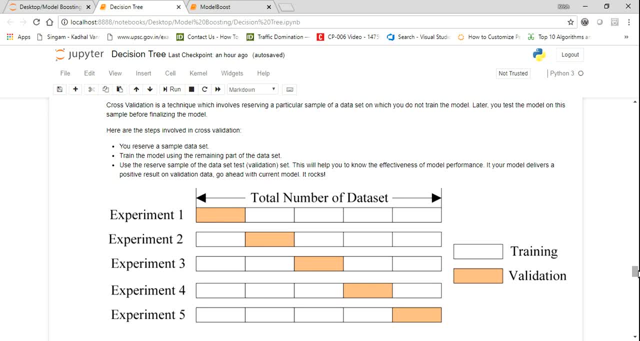 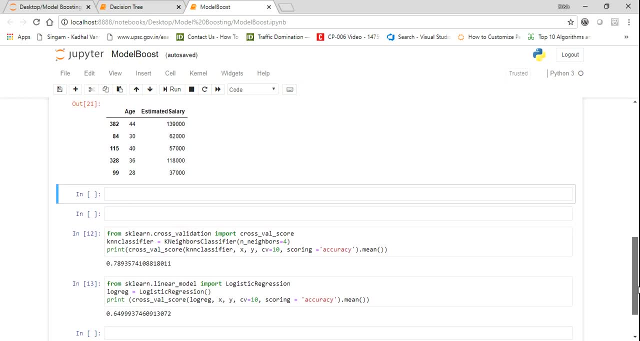 good results And I hope the accuracy will also be increasing. Now let us see how we can implement this cross validation in Python by using sklearn. So, to implement the cross validation, I'm going to import a library from sklearncrossValidation, a library named as crossValScore. 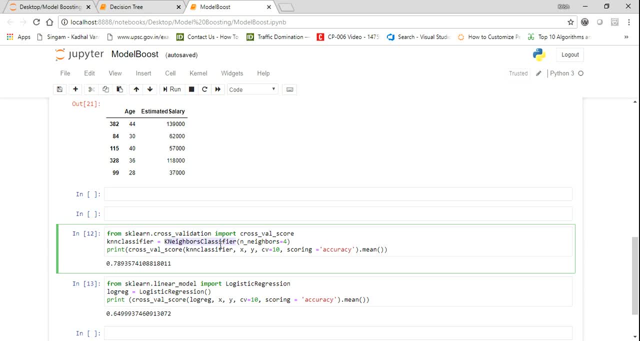 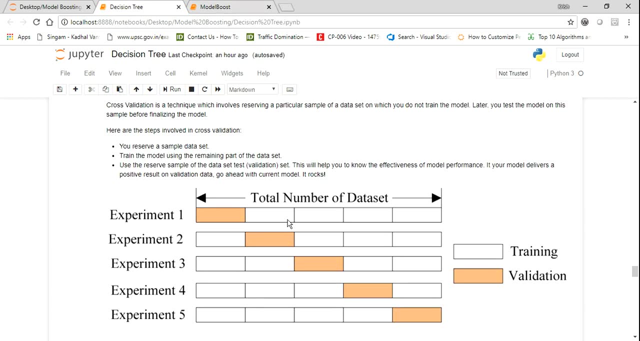 Again, In the first case, I'm going to use the k nearest neighbor classifier and the n neighbors is basically four. Now what we are going to do is that, if you want to implement this particular technique, we will be calling this cross ValScore. 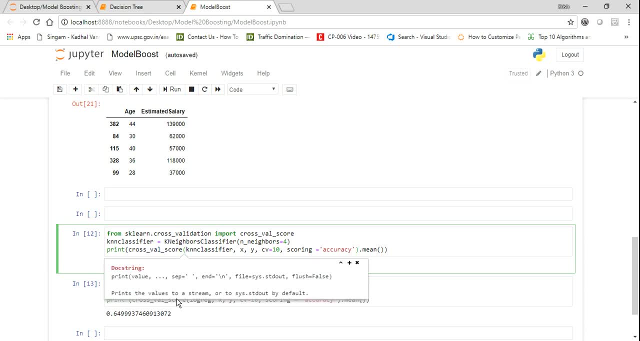 In that cross ValScore the first parameter is basically: this is the print method. What I'll show. let me show you the parameters that are involved in this cross ValScore. Okay, So if you see the first parameter in cross ValScore by pressing shift tab. 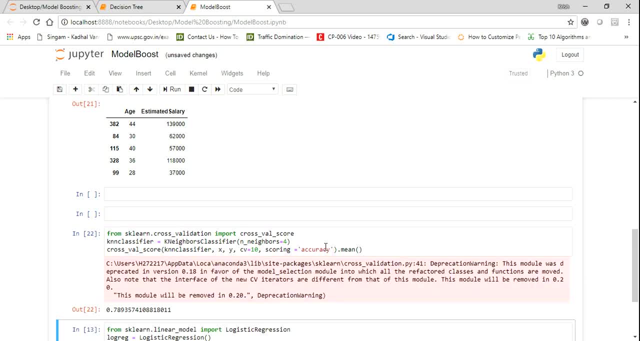 Let me just execute this once. here it is. So we have getting a warning. It says: model selection. Okay, Let's use model selection instead of cross validation. So model selection, and let's press shift tab. Now you can see that the first parameter is basically the estimator. 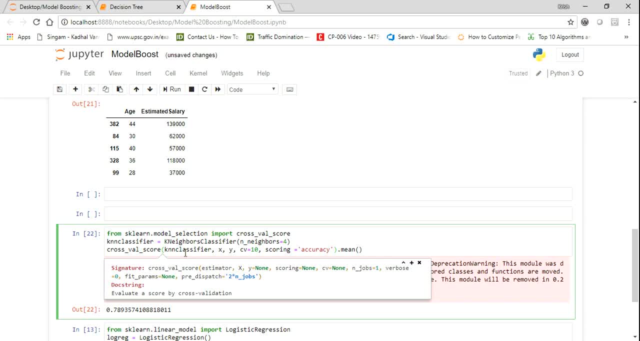 The estimator basically specifies that which machine learning algorithm we are going to apply, So it is nothing but KNN classifier. The second and third parameter are: basically: we are providing the S test, X data and Y data, which is nothing but the independent and the dependent variables. 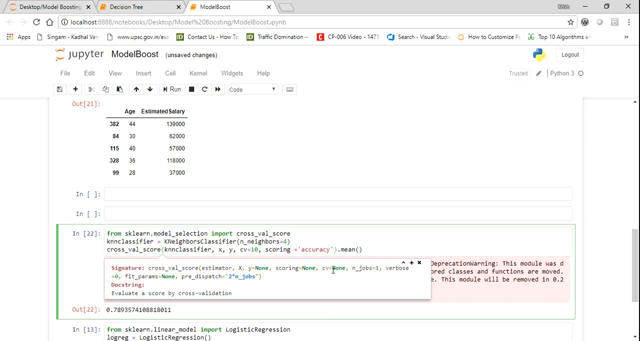 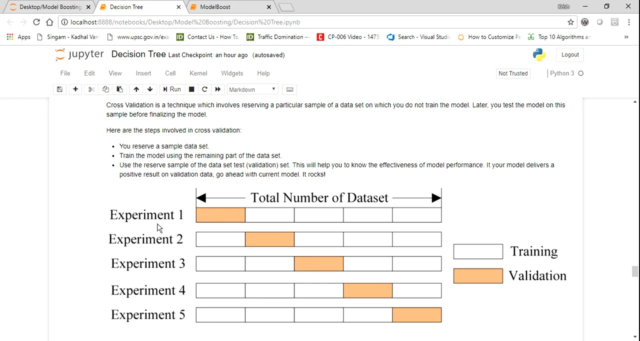 The third parameter is something called as CV. CV basically means that cross validation. Now, what is the value that you need to specify in CV? Okay, Suppose if I take this example, okay, if I have 25 rows of data and if I complete like: 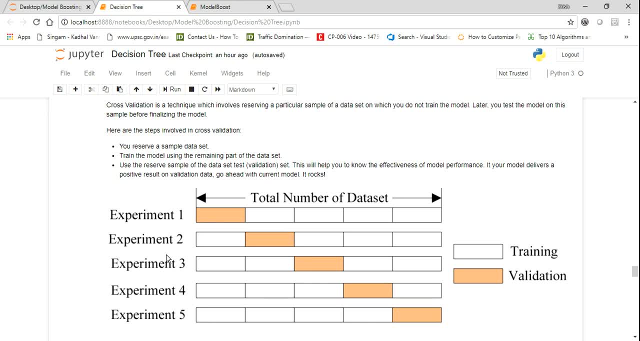 five different experiments, Or five K-folds. this is also called as K-folds. okay, Once I do this, five K-folds- in this case, the CV value actually will be five. So this completely depends on the type of folds that you want to do with respect to. 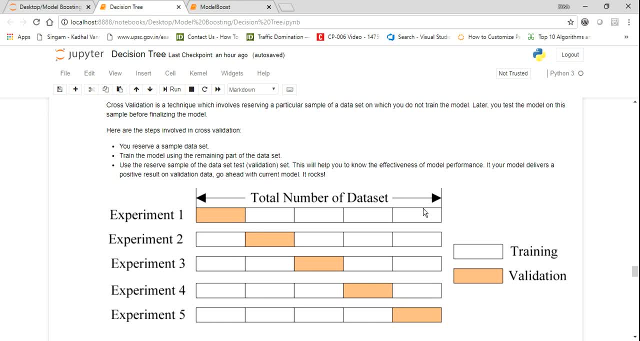 the data. Okay, Now suppose, if I have 25 data and if you want to do five folds, that basically means that that 25 data will be divided by five And in that case your test data will be actually five and the remaining data will be your training. 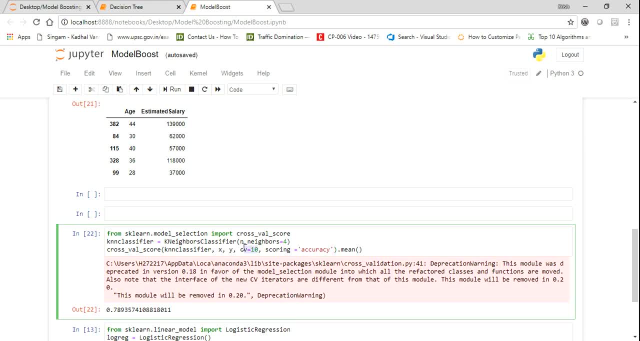 So let us do one thing. Let us just select the value, as CV is equal to 10, okay, Once I select, the CV is equal to 10 and my scoring is basically accuracy. What it will do is that the KNN classifier will directly compute the scoring for accuracy. 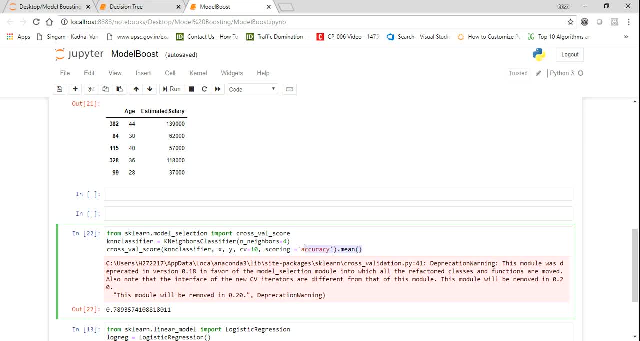 level for us, And then we are going to apply the mean of all the different kinds of scores that we will be getting. So before executing dot mean, let us see 10 different experiments gives us what? all kinds of results. So I'm going to print this: 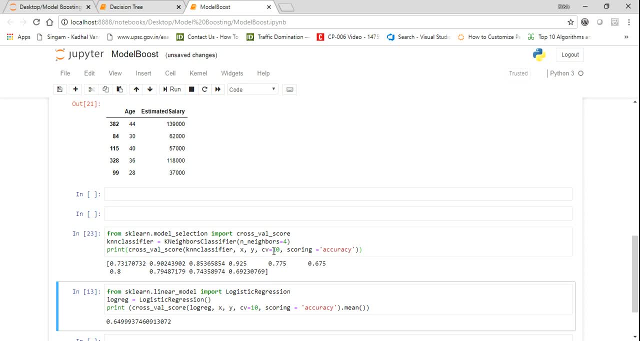 Okay, And let's see the value. Now you can see that, since I've given, CV is equal to 10. for the first experiment, I'm getting 73% of accuracy. For the second experiment, I see that I'm getting 90% of the accuracy. 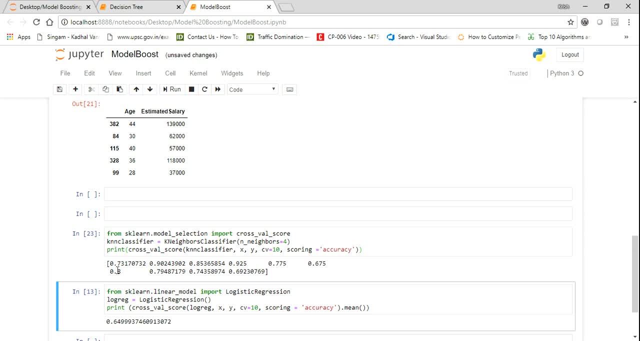 For the third experiment: 85,, 92,, 77,, 67,, 80,, 79,, 74 and 69.. So what we can do is that now all these accuracy mean can be taken And finally we'll be able to get them final accuracy. or it says an invalid syntax because 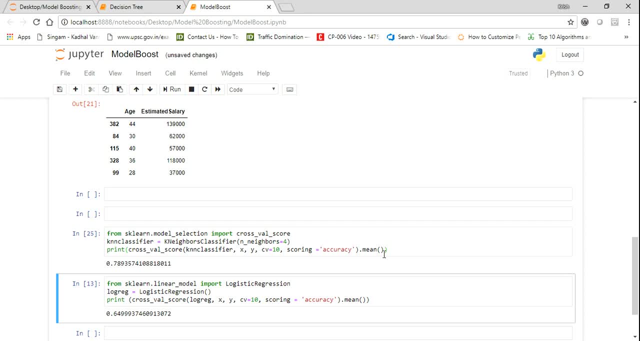 I did not write dot, So once you do the mean, you will be able to get a very good accuracy of 78%. Now, please note that this is with different type of training and test data set. Okay, Now we have actually used K-nearest neighbor. 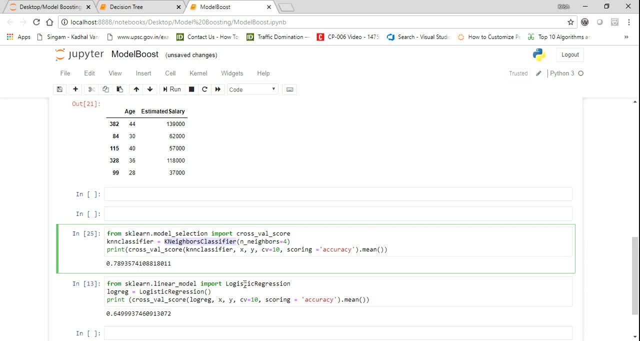 Can I apply different kinds of algorithms or classification algorithms? For an example, if I take logistic regression and I apply the same process instead, the estimator is getting changed to log rec, which is the object that I've created here. Again the same thing. 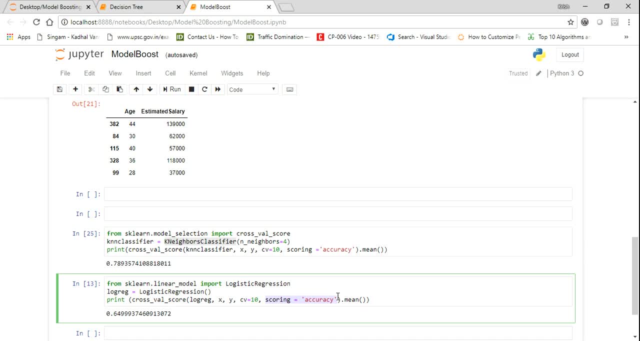 I've selected, CV is equal to 10.. I'm going to see the squaring is equal to accuracy and I'm going to do it as dot mean. Now let us see the accuracy that we are getting. We are getting 64%. So this basically means that the cross val score, since the data is completely different. 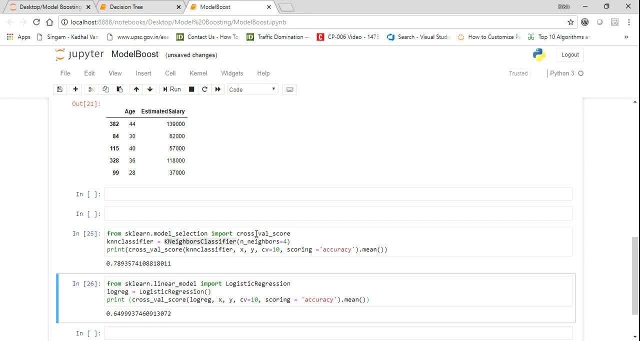 now the training and test data set is differing based on the experiments that we are doing. Suppose, if I'm giving CV is equal to 10, that basically means that 10 different experiments we are doing And for each and every time the training and test data set is actually different.